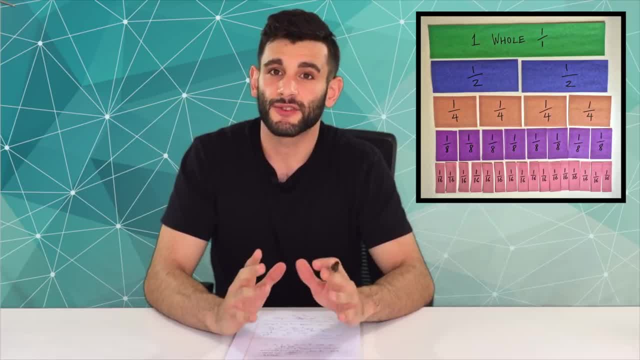 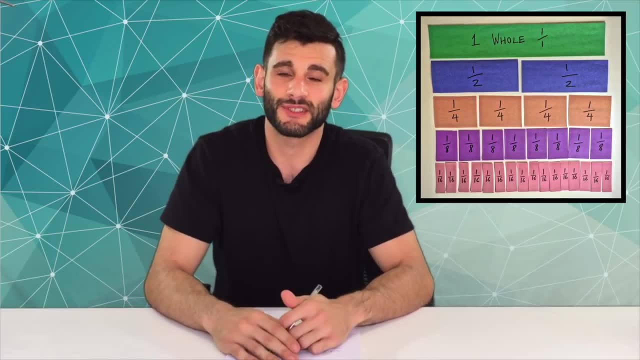 a fraction kit And the reason why I chose this activity for the first episode. it's pretty simple, but it's very powerful. I used to do this with my middle school students and I wish I would see more teachers doing this, but there's. so maybe something you want to add to your repertoire of. 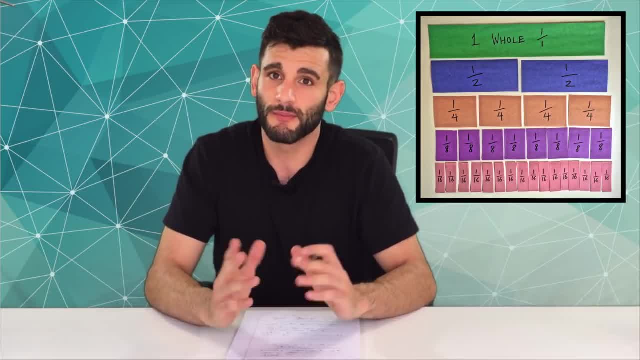 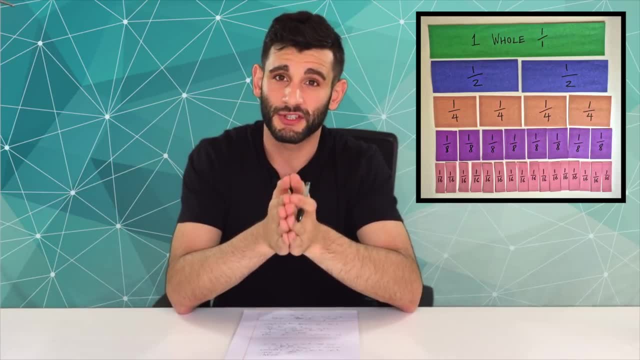 teaching activities, especially if you work with elementary or middle school students. So we want to get a good, strong foundation of fractions as soon as possible, and activities like this help us to achieve that goal. I just want to quickly remind you before we start that there. 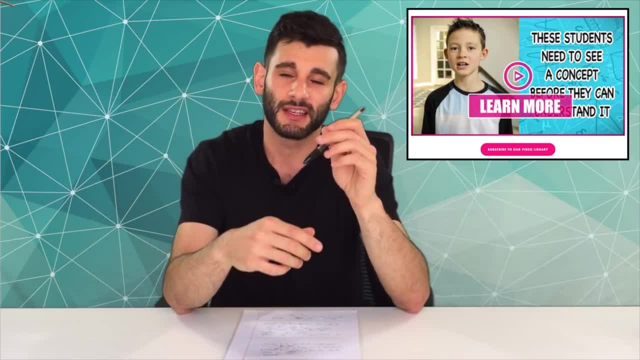 is a worksheet that accompanies this lesson. You can download it for free. It's on mashupmathcom. The link is in the description. So if you're new, welcome. And if you're new, welcome. And if you're new welcome, The link is in the description. for this video, You don't need the worksheet. 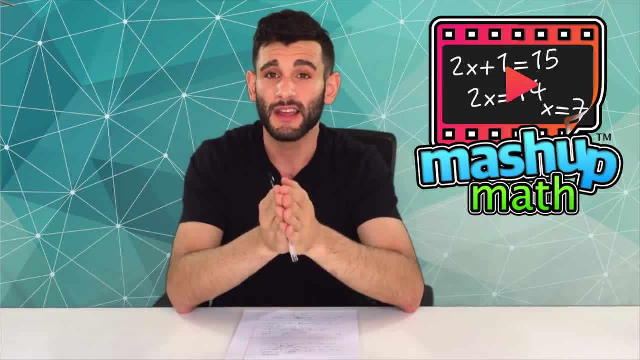 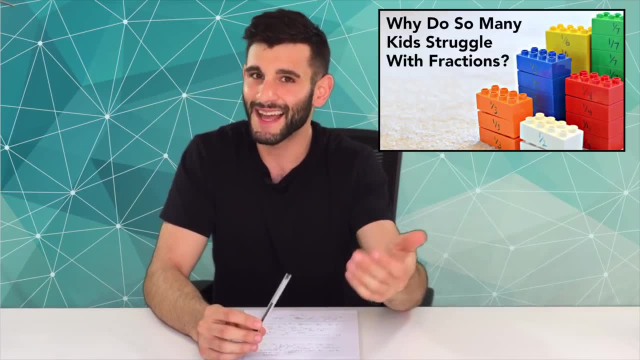 but if you want something to follow along as you go through the activity, then you can definitely do that, And I've also written a blog post, which is also on mashupmathcom, where you can get some more insight into this activity and the research behind why activities like this help students. 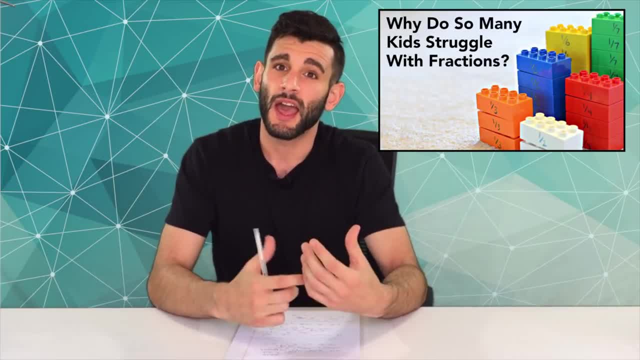 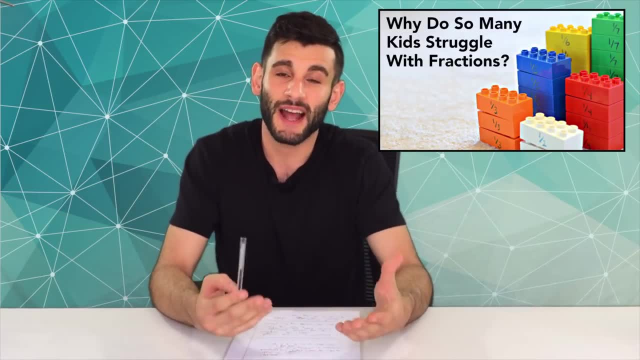 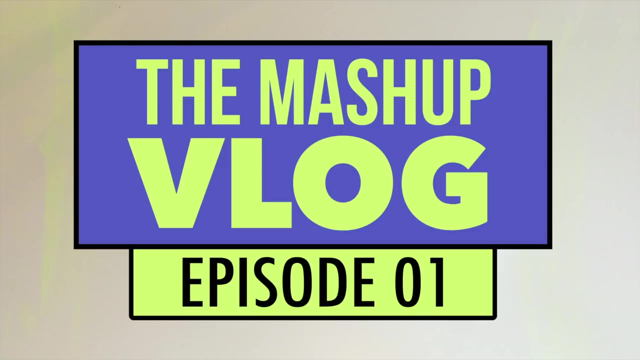 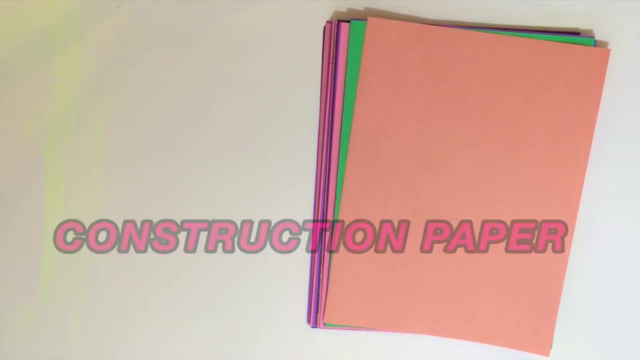 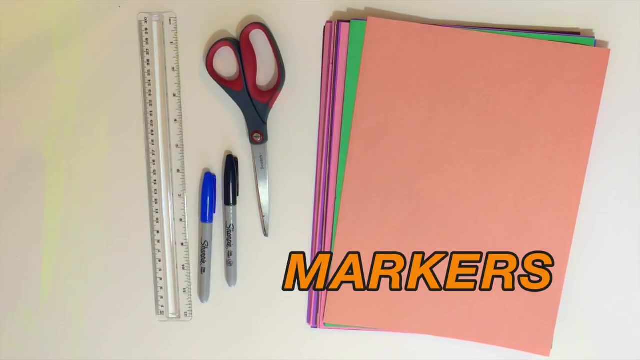 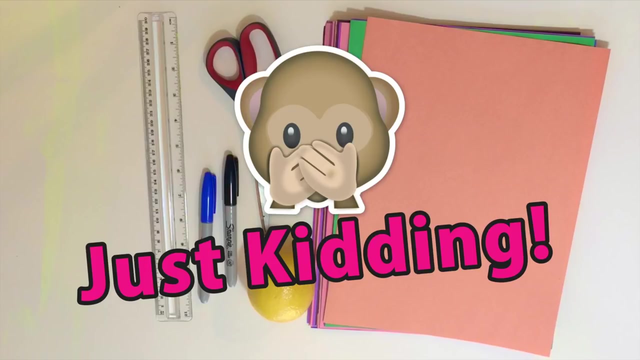 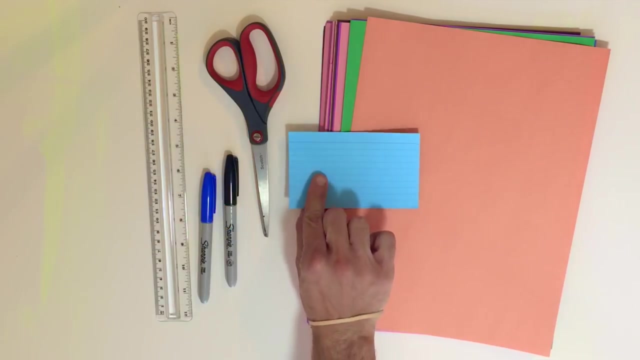 to gain a conceptual understanding of a math topic and why we want to avoid things like just simply memorizing definitions and doing a lot of robotic repetition. In practice, it's about understanding, and activities like this help us to do that. The link is in the description, So if you're new, progress and learn how to do that. 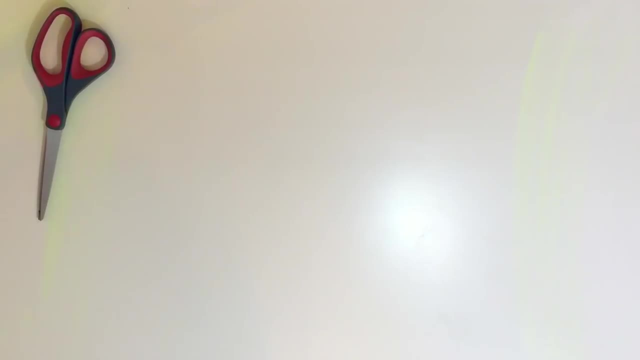 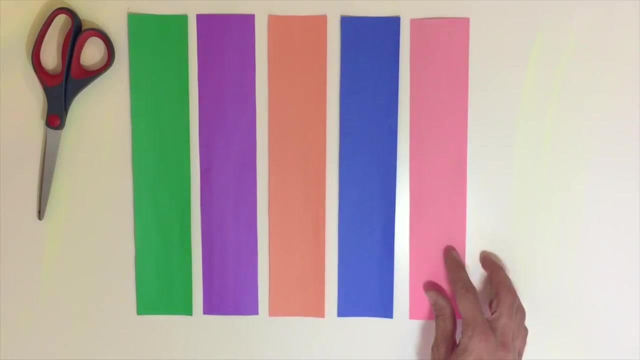 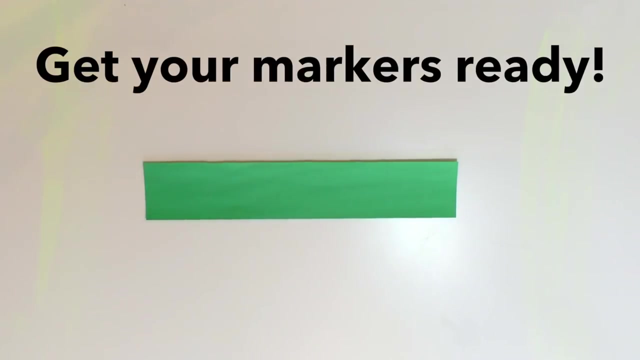 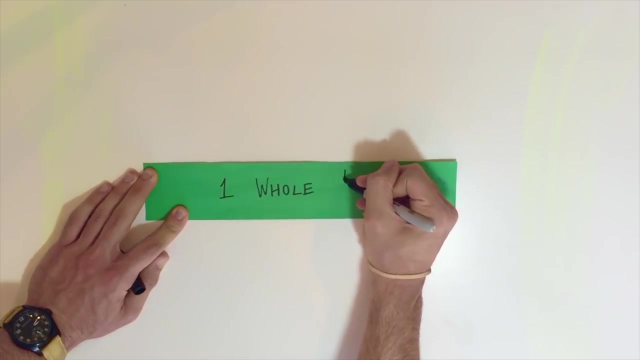 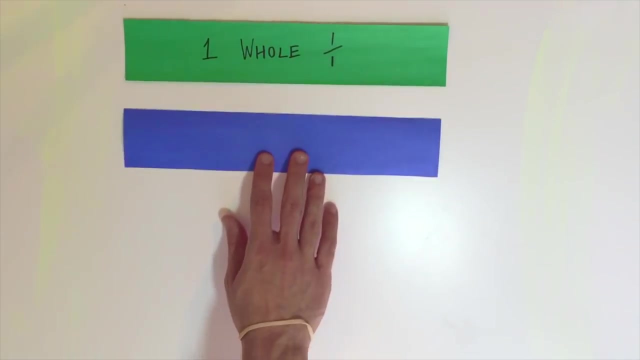 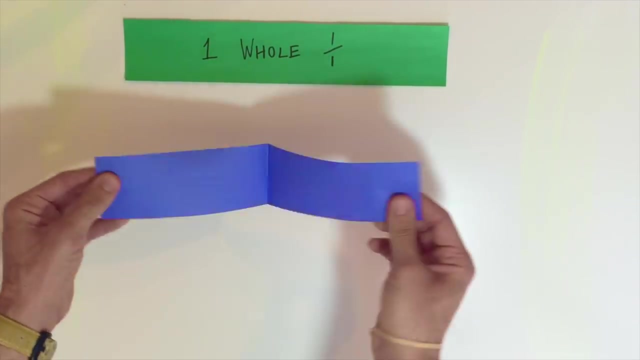 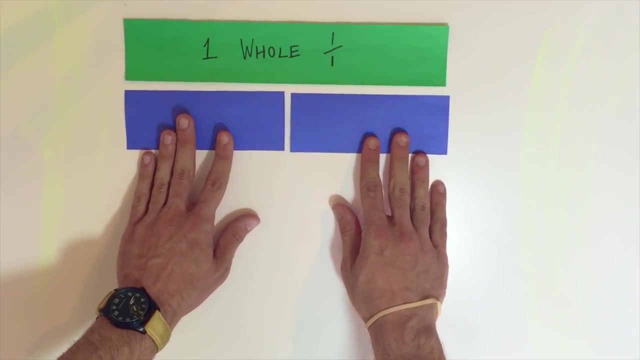 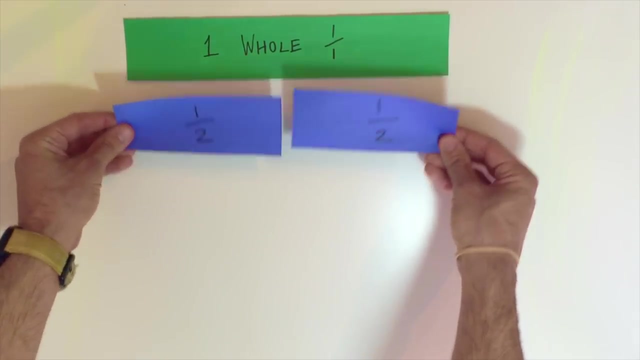 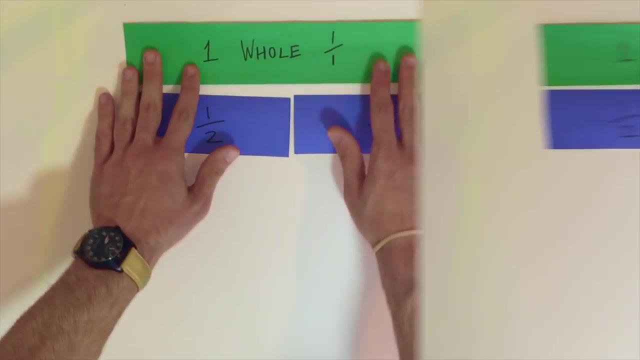 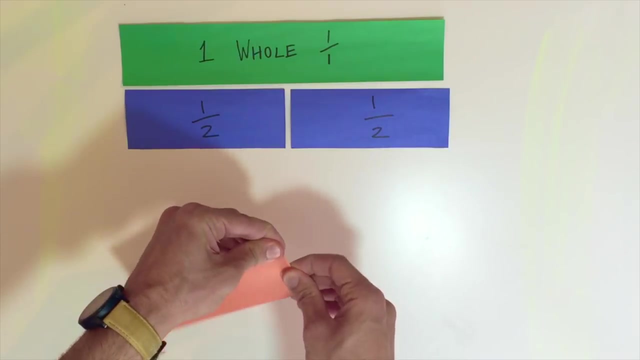 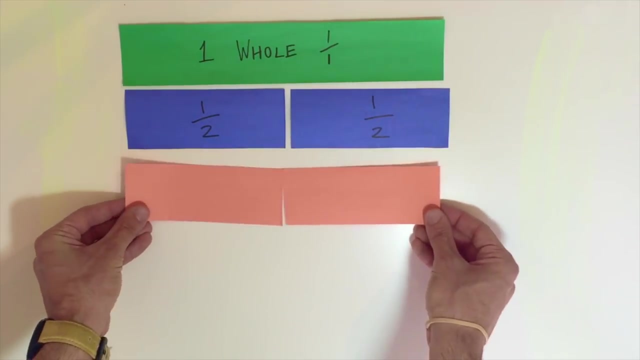 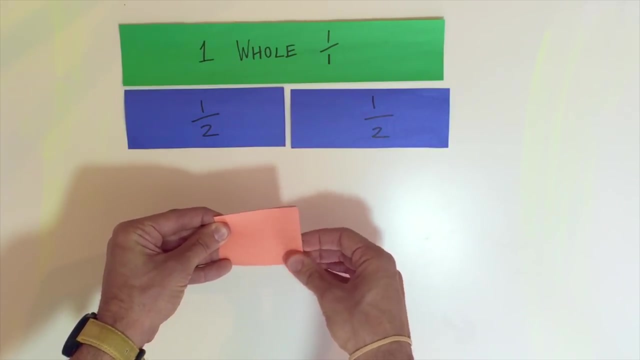 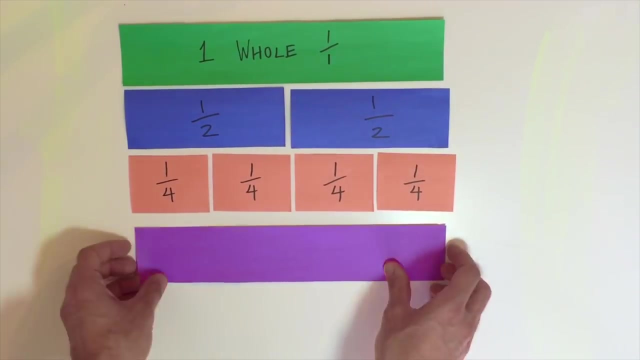 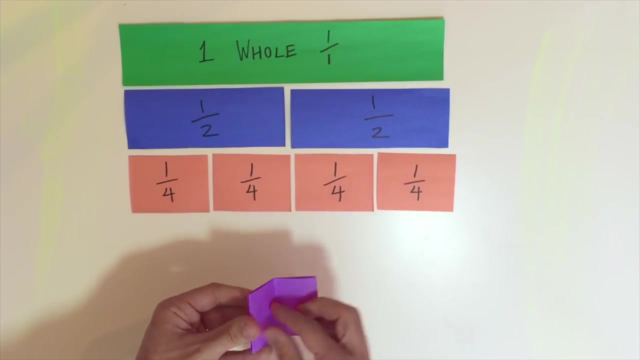 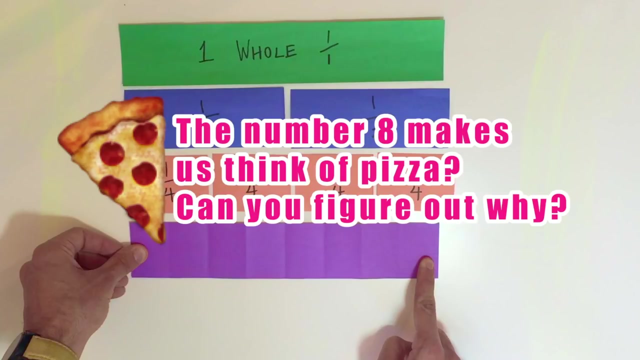 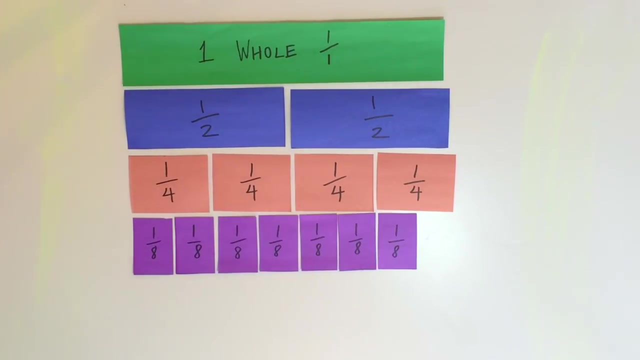 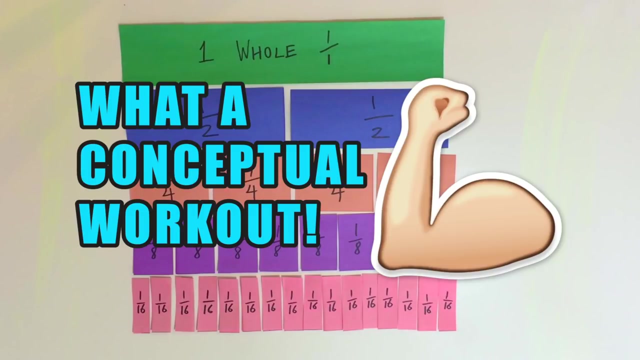 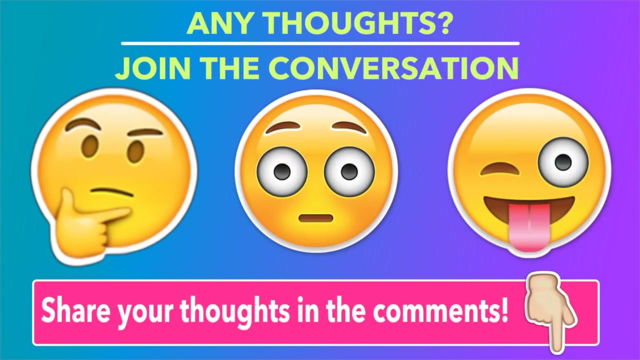 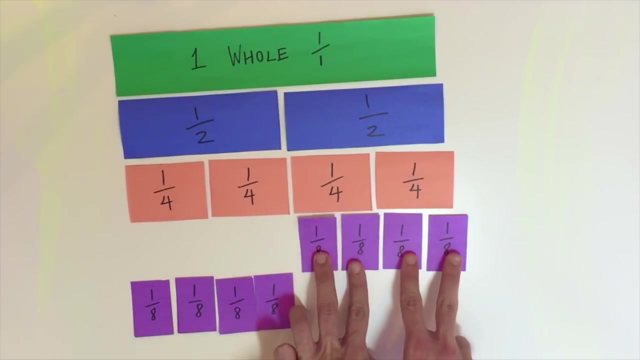 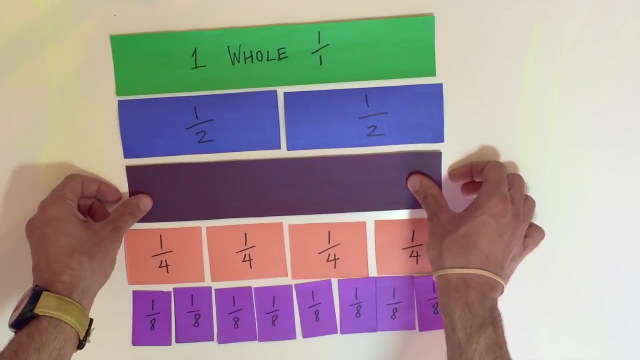 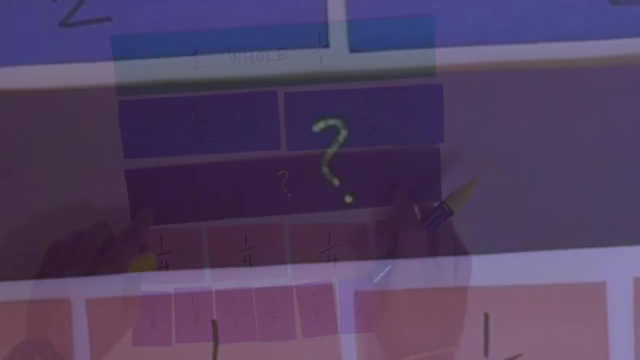 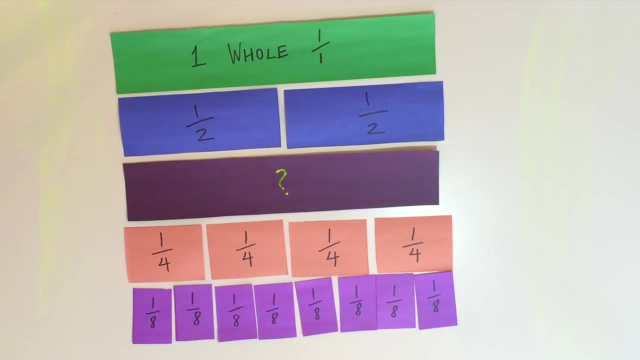 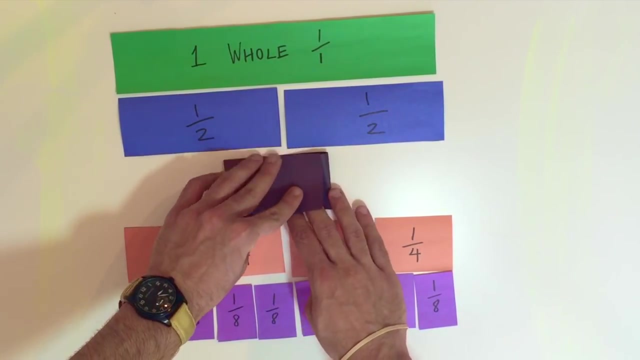 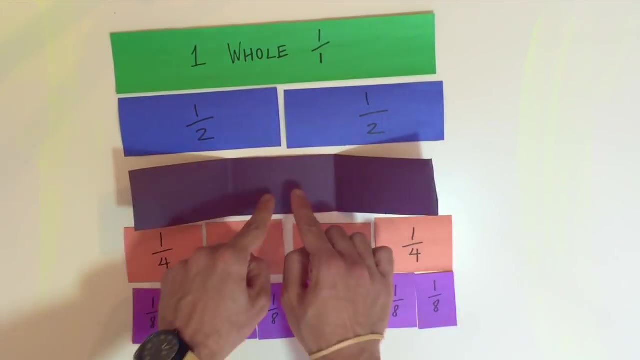 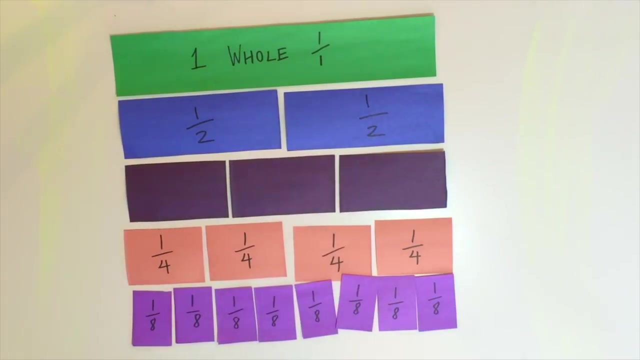 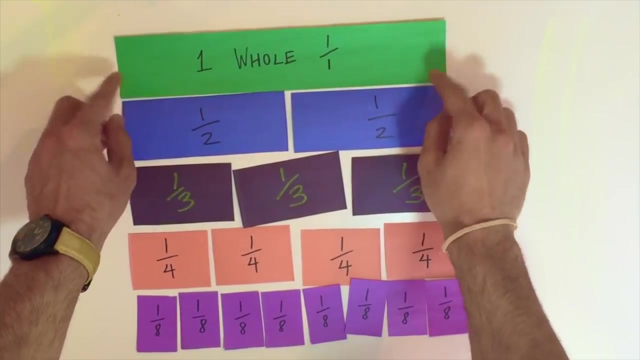 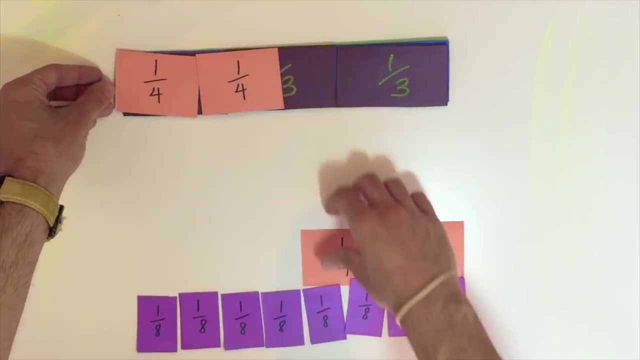 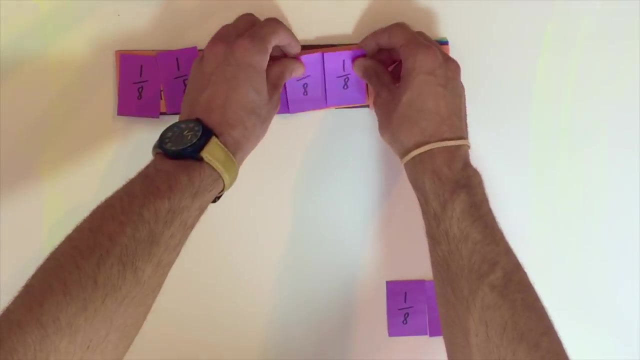 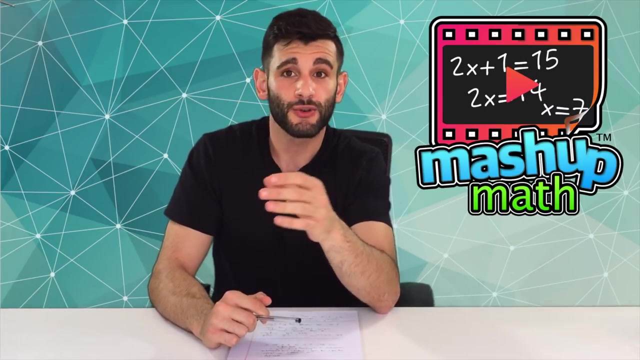 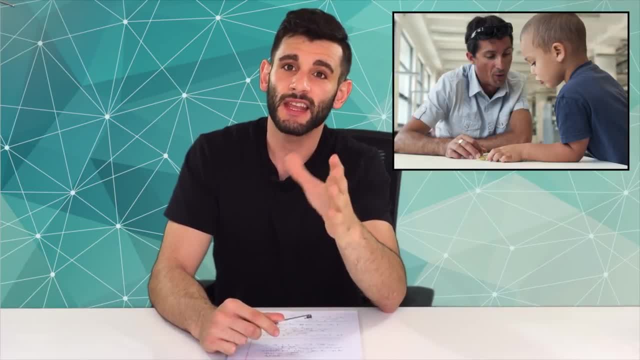 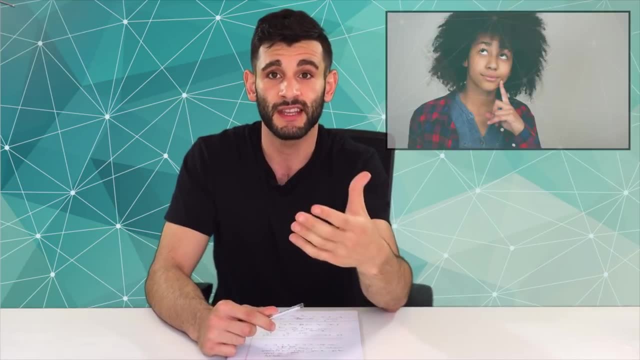 This is an exploratory activity, And what I mean by this is that if the student is struggling or making mistakes, allow them to make those mistakes, It's okay. This is an exploratory activity. Let them explore, Let them mess up. 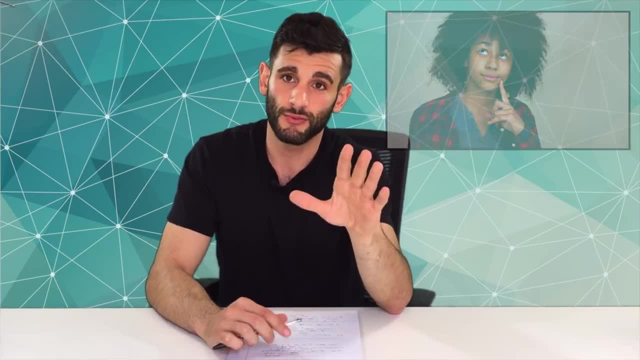 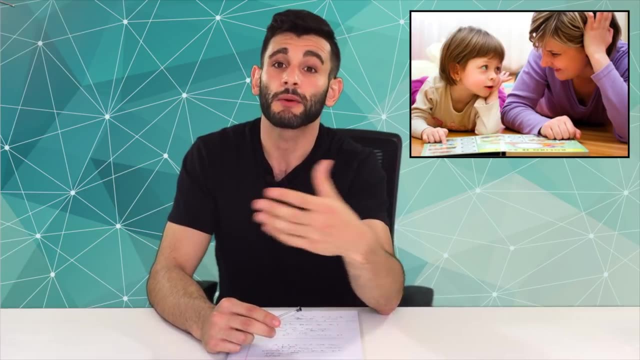 Then whatever they're doing wrong, let it happen. Okay, don't rush in to correct them, because they might correct themselves, And if they don't, you can wait till later on to have a discussion or to explore why what they were doing was incorrect. 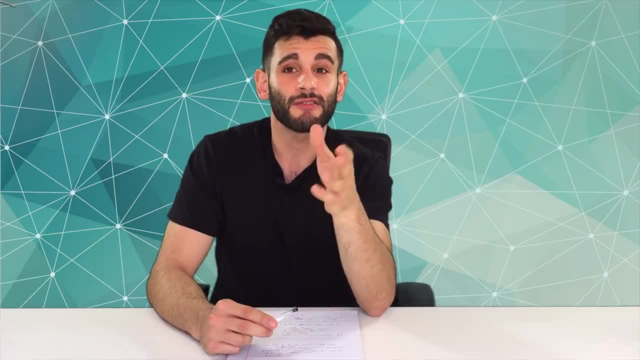 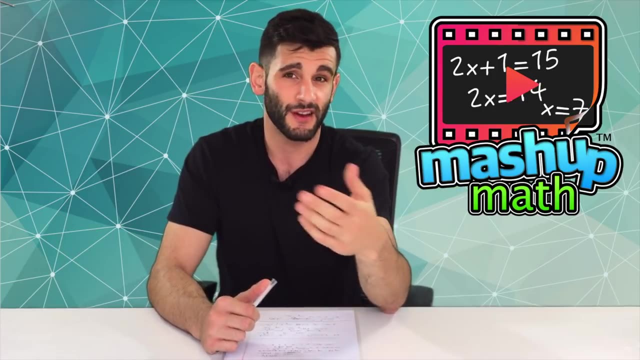 And then let them explore more in the right direction. And again, remember there is a worksheet that goes along with this lesson. You can be really creative with this. You can add new questions, new fractions, throw some curveballs in there. 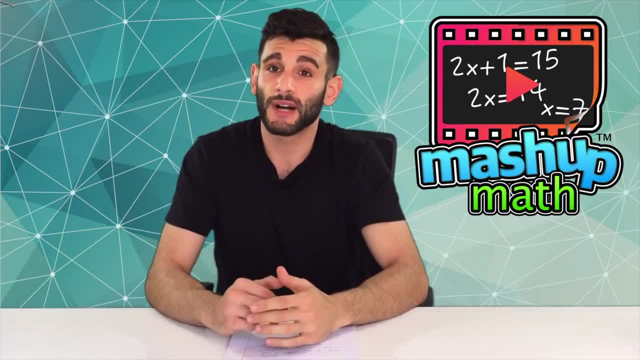 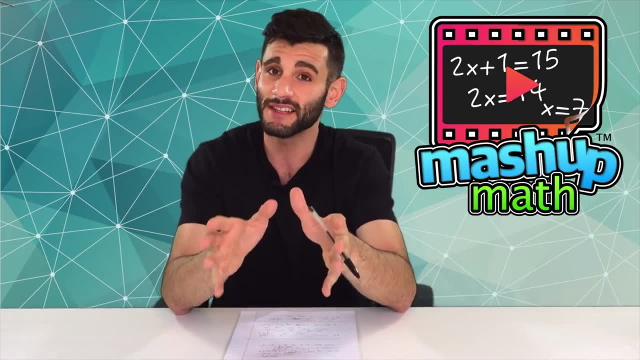 Customize it any way you want, Take it and run with it, And if you have some cool ideas, I would love to hear them in the comments section below this video. And finally, I want to share with everyone that Mashup Math is committed to sharing free and accessible math resources. 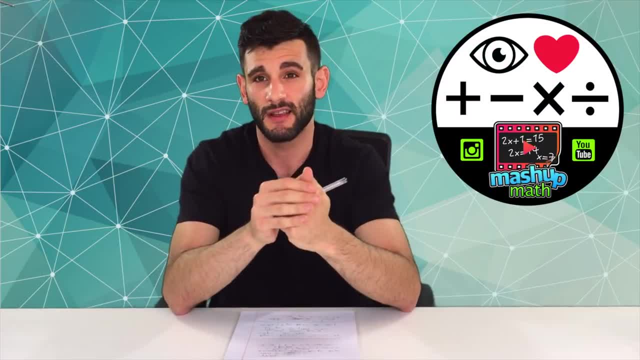 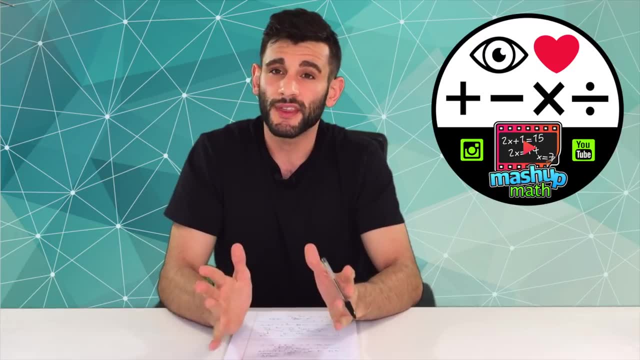 because we want to reach as many students, schools, teachers, parents as possible. So, with that in mind, if you want to support us, if you find what we're doing to be helpful, you can do a few things that take very little effort and would really help us out. 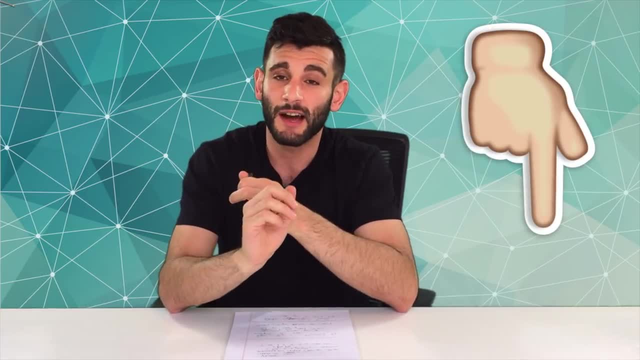 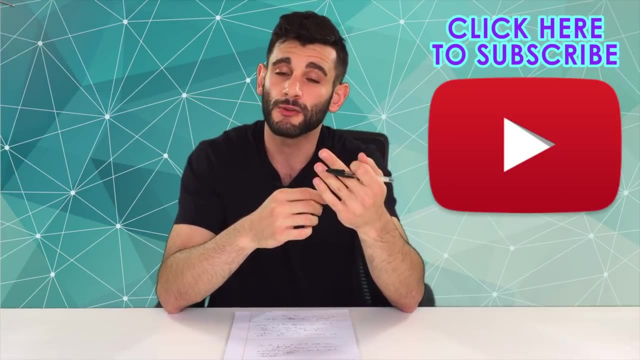 One of those things is to like this video. A second thing is to leave a comment in the comments below. If you like the video, let us know why. If you have questions- comments concerns- The third thing you can do is subscribe to our YouTube channel if you're not already. 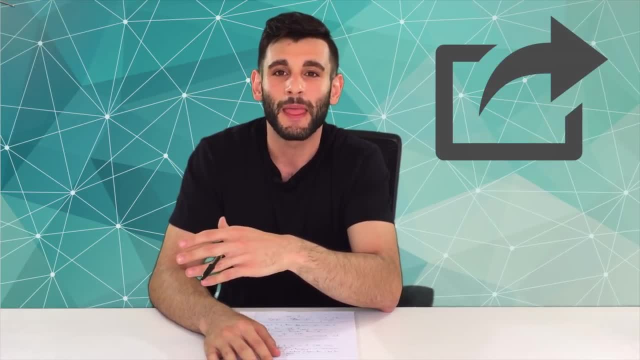 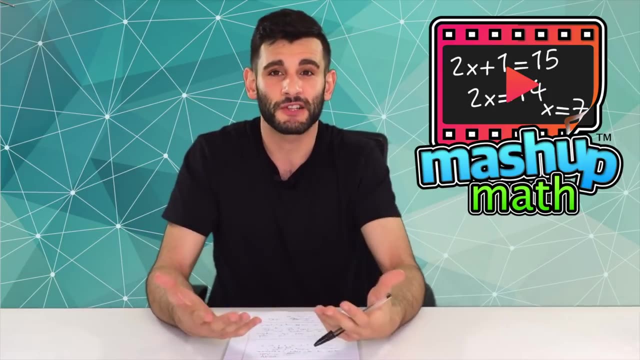 And the fourth thing you can do is share this video on whatever social media outlet that you prefer to use, So Facebook, Pinterest, Instagram, Twitter- wherever Sharing it helps to boost our exposure and makes it easier for us to attain our goal of reaching as many students as possible. 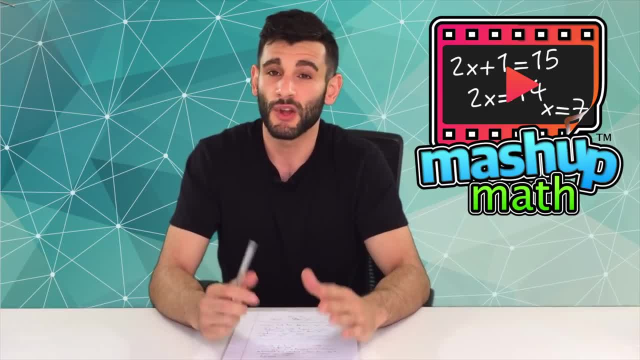 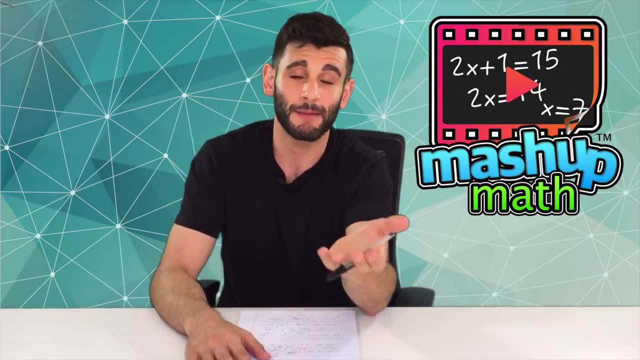 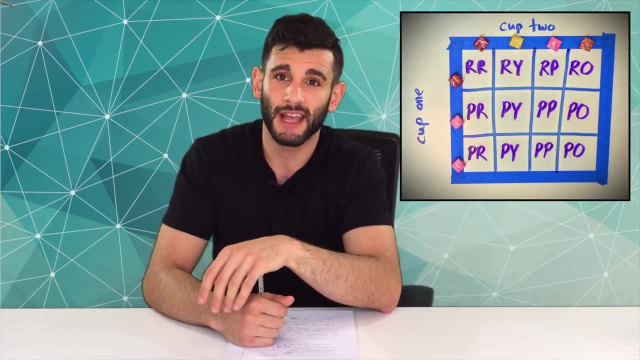 So one of those four things, all of those four things, any combination would mean a lot to helping us out. So, on behalf of the whole team here at Mashup Math, Thank you all for checking us out And come back. next Thursday will be episode number two, which is going to focus on area models for analyzing probability outcomes. 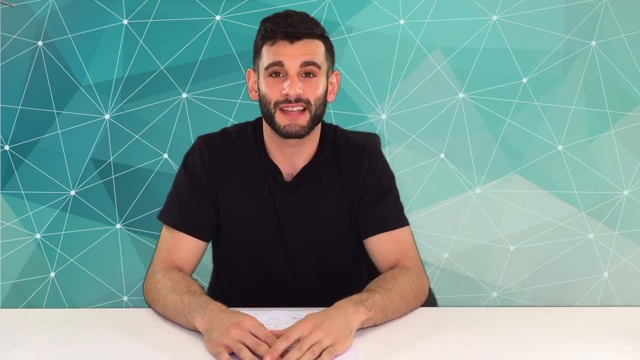 Another pretty cool activity, So you won't want to miss that. So thanks a lot and we'll see you next time. 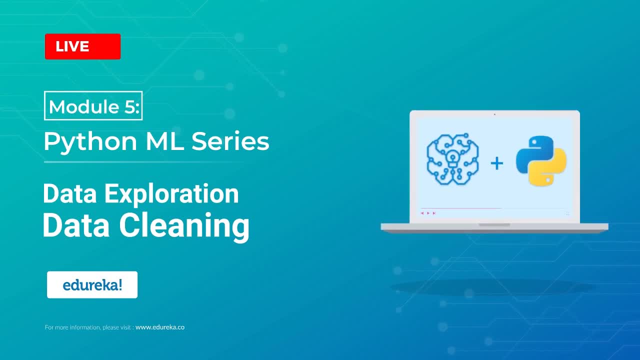 Hello everyone, This is Vasim from Edureka, and I welcome you all to this session, which is the part 5 of the python ml series that we are making. in this session, We are going to talk about how we are going to clean our data.